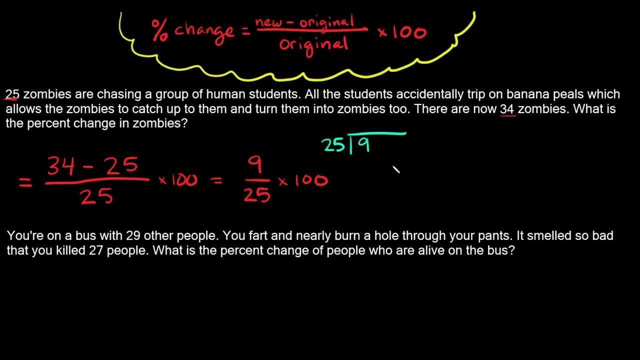 divided by 25.. Okay, as you can see, 25 doesn't go into 9, right? So what we have to do here is put a decimal point and a 0.. Okay, now you ask yourself: does 25 go into 90?? Well, yes, it does. 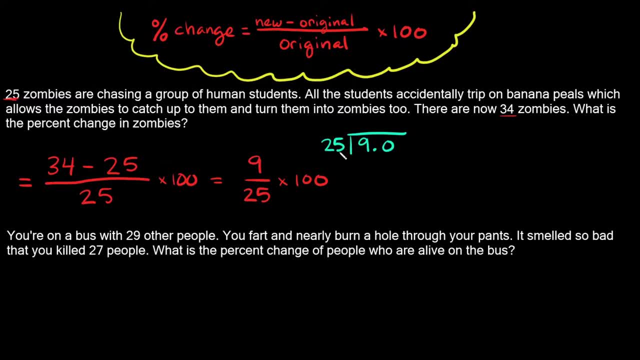 How many times? Well, whenever you're counting by 25s, an easy way of thinking about it is thinking of quarters, right, Like with money. So, if you have one quarter, you have 25 cents, right? If you have two quarters, you have 50 cents. If you have three quarters, you have 75 cents. If you have 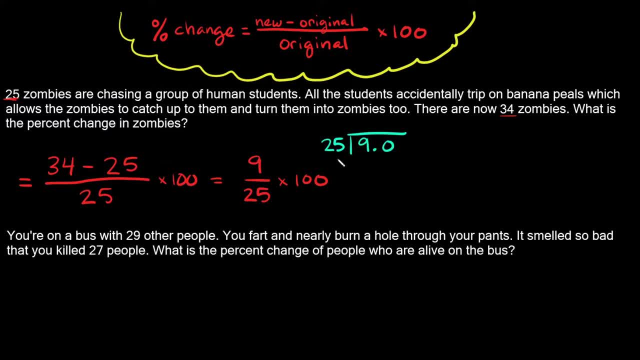 four quarters, you have 100 cents, or in other words a dollar, right? So in this case, 25 goes into 90. three times okay, And then 3 times 25.. Or again, three quarters is the same thing as 75 cents, or just 75. Okay, so then you have to. 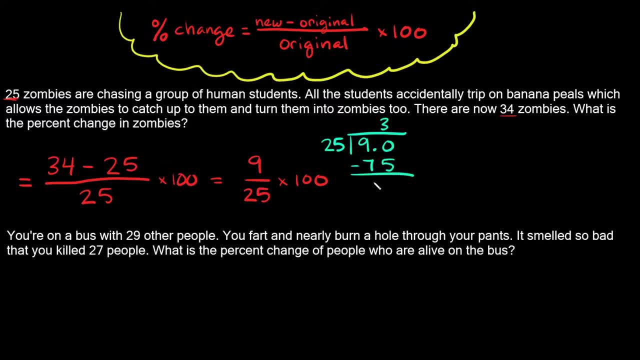 subtract here 90 minus 75,, which is equal to 15.. Okay now, we don't have a number over here, So we'll put a zero so we can bring that straight down. Okay now, how many times does 25 go into? 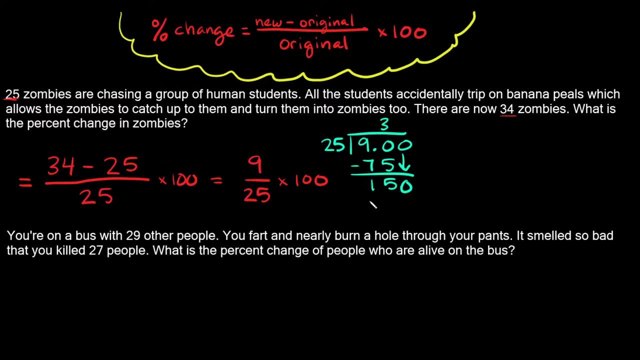 150? Okay. or again, the other way you can think about this is: how many times does 25 cents fit into a dollar 50?? So 25 must go into 150, exactly six times, Okay. so then, six times 25 is 150.. You subtract and you. 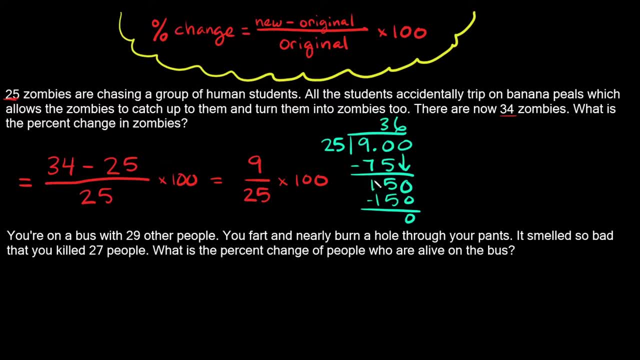 get no remainder. Okay, so this is almost our final answer. The last thing you have to do is grab your decimal point and bring it straight up to your answer. Okay, so your answer right here would be 0.36. Or, more properly written, it would actually be 0.36.. Okay, so nine over 25 is. 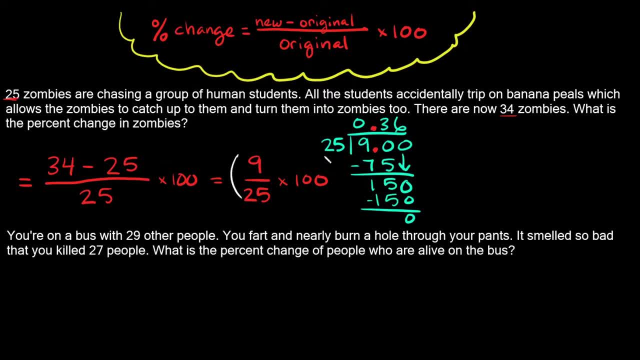 equal to 0.36.. Okay, so I'm going to write this right here, but with the decimal now. So this is now equal to 0.36 times 100.. Okay, so now we're just multiplying by 100 in order to change this. 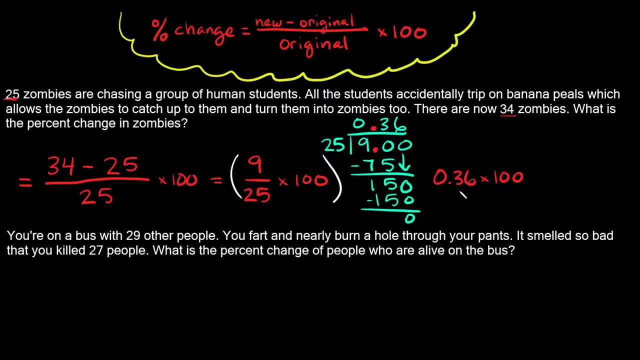 decimal into a percent. So what is 0.36 times 100?? Well, an easy way of multiplying by 100 is just realizing, since you have two zeros, right. So you're going to multiply by 100 times 100.. Right here, you just have to move the decimal two times to the right. Okay, so one, two, So that's. 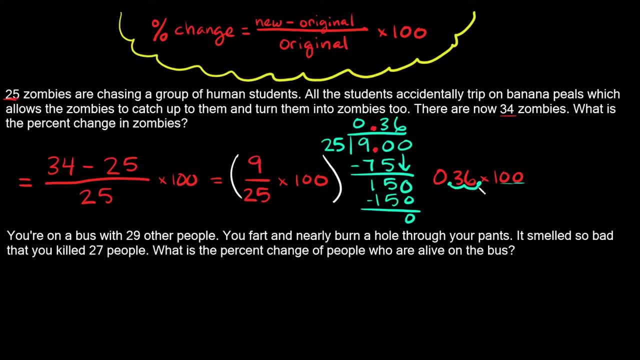 where your decimal is. So instead of having 0.36, this is now going to turn into 36.. Okay, so this is going to be equal to 36%. So again the question was: what is the percent change in zombies? 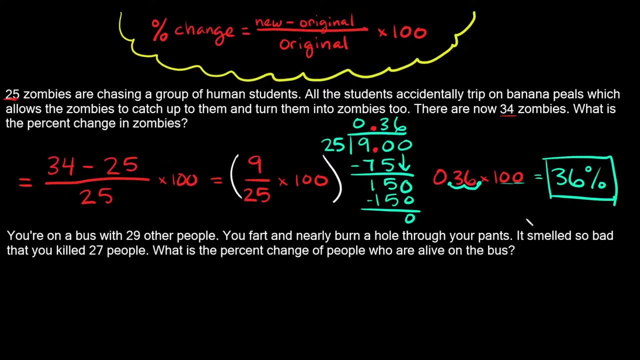 And your answer would be 36%. And also, since we got a positive number for our answer, right, positive 36%- that means there was a percent increase, All right, so hopefully that wasn't too bad. Let's do just one more example, All right. 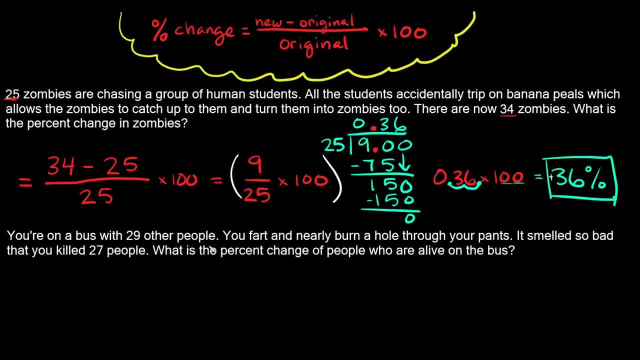 so this problem says you're on a bus with 29 other people, You fart and nearly burn a hole through your pants. It smelled so bad that you killed 27 people. What is the percent change of people who are alive on the bus? 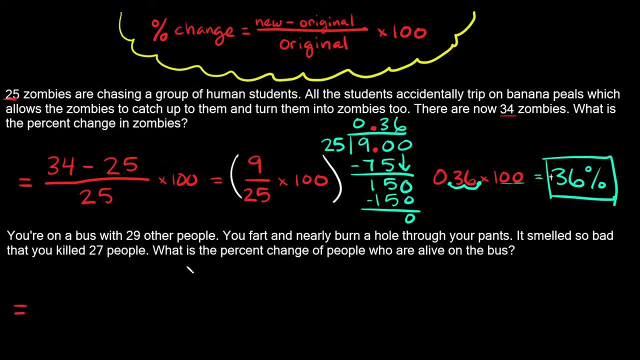 Okay, so let's get a couple things straight. So the problem is asking: what is the percent change of people who are alive? Okay, so originally, how many people were alive on the bus? Well, you started with: you're on a bus with 29 other people, right? So it's you plus 29 other people. 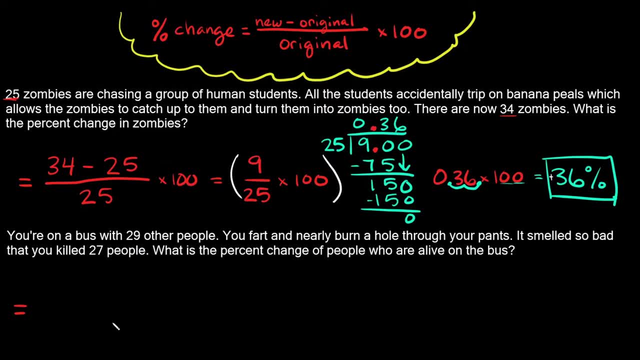 So that means there were originally 30 people who were alive on the bus. Now you farted and you killed 10 people. So what's the percent change of people who are alive? 27 of them, right. So now, how many people are alive on the bus? Well, that would simply be. 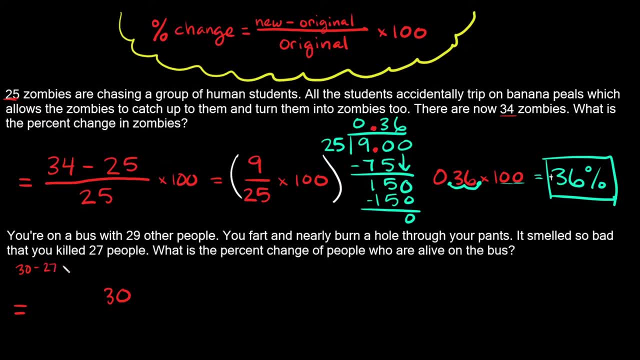 30 minus 27.. What is 30 minus 27? 3.. Okay, so now there's only 3 people who are alive on the bus, So that means your new amount of alive people would be 3.. So, following the formula, the percent change is equal to the new amount of alive people: 3,. 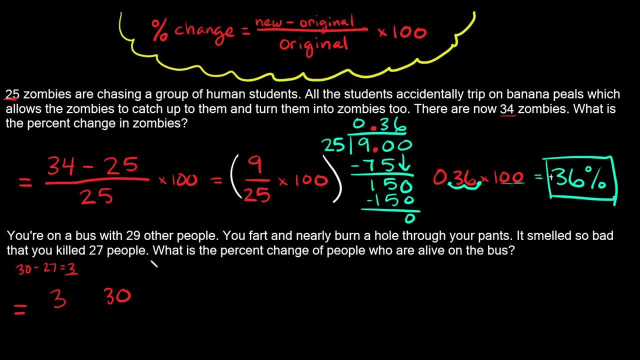 minus the original amount of alive people: 30. Okay, so, 3 minus 30. And then we're just going to divide that by the original amount of alive people, which again was 30. Okay, so we're gonna simplify this and then just multiply by 100 at the end. 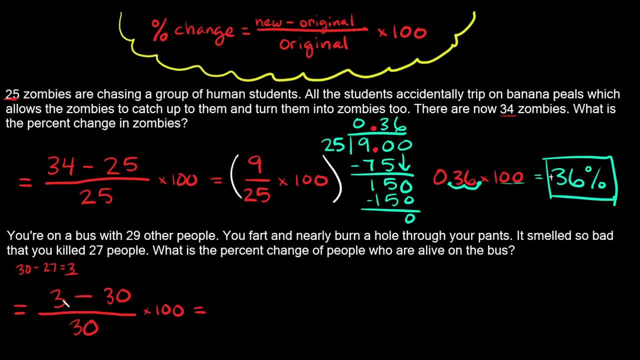 Okay, so this is going to be equal to. now, what is 3 minus 30?? Well, that would be negative 27,. right, And because you have a small number and you're subtracting away a bigger number and then that's going to be over. 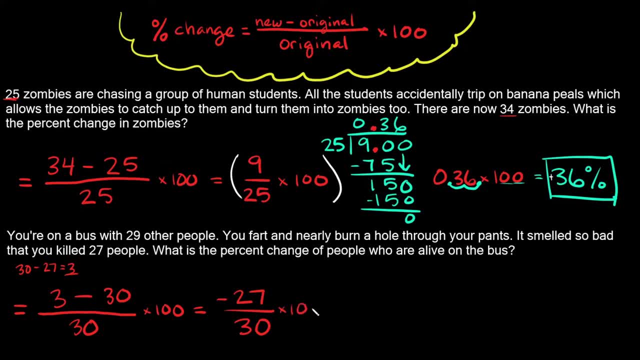 30. And then again we're just multiplying by 100.. Now, can we simplify this fraction anymore? We actually can, right, Because we can divide the top and the bottom by 3. Both of these numbers are divisible by 3.. 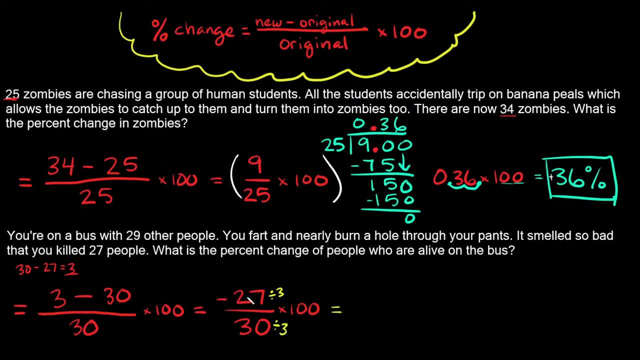 So then this is going to be reduced. So what's 27 divided by 3?? 9,, right, And remember it's negative: 9, right, Negative, 9.. And that's going to go over 30 divided by 3,, which is 10.. 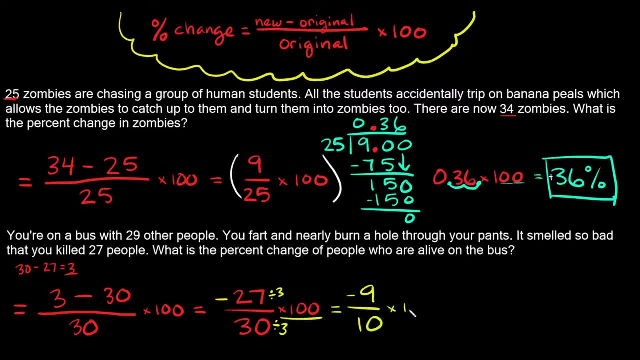 Okay, and remember, we're multiplying by 100, right Times 100.. Now this problem we can solve the same way we did the last one. okay, We could turn this fraction into a decimal and then multiply it by 100.. 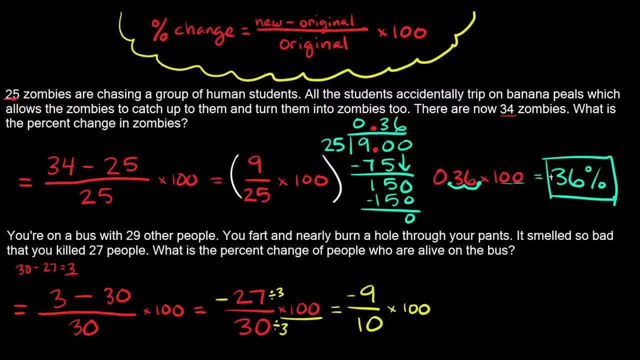 But in this case we can actually do this a little quicker, okay, Because we can just multiply this fraction times 100.. Okay, so how do you multiply a fraction times a whole number? Well, an easy way of doing that is simply turning the whole number into a fraction, okay. 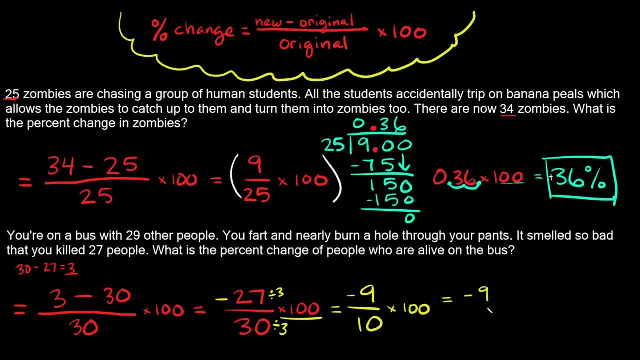 So I'm going to rewrite it like this. So I'm going to say negative 9 over 10 times, and then how do I turn 100 into a fraction? Well, I just have to put it over 1, right, 100 over 1.. 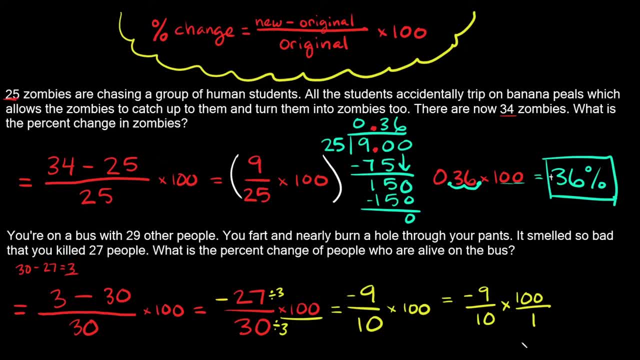 Okay, so now here we just have a fraction times a fraction, right, And in order to multiply fractions together, you just multiply straight across, right? So you multiply the top together and multiply the bottom together. But one thing I'm going to do before doing that is simplify this a little bit, And the way I'm going to do that is by